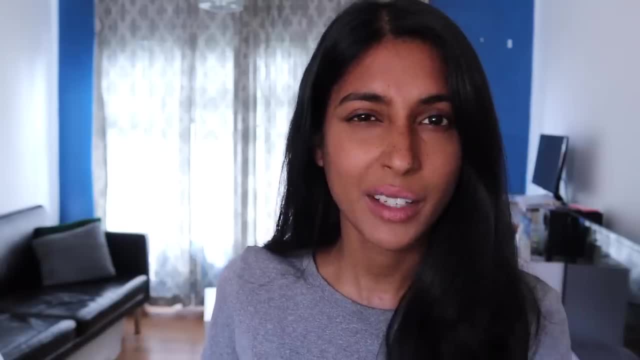 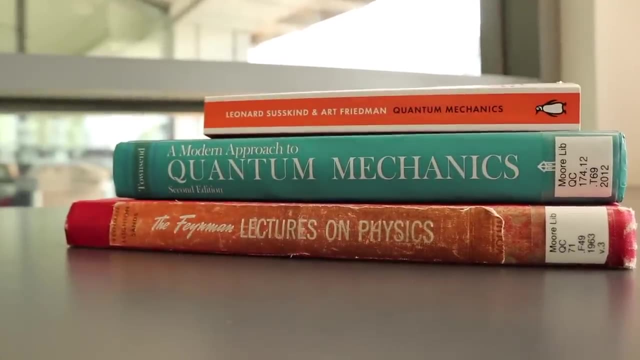 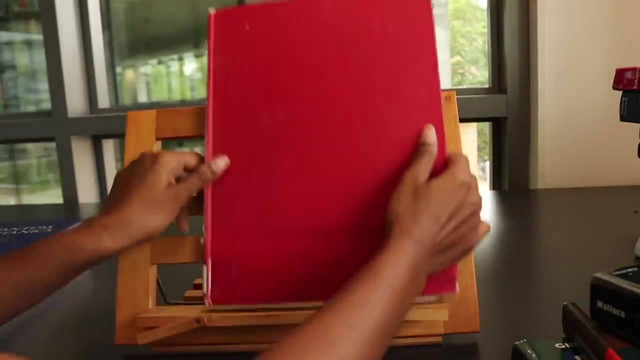 And a lot of popularizations of quantum mechanics are kind of useless because they just rely on analogies. But there are some good resources in between, And so I made this video to recommend some of them to you. Let's start at a book that I would recommend to everyone, from complete. 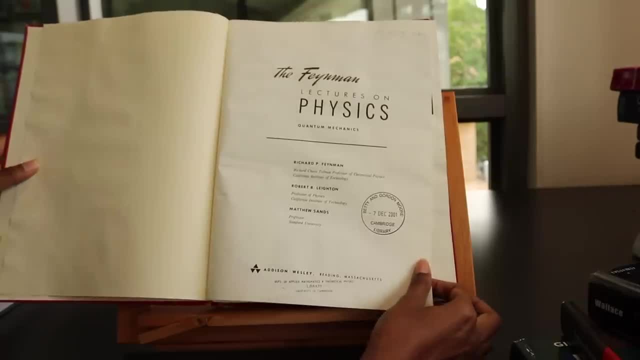 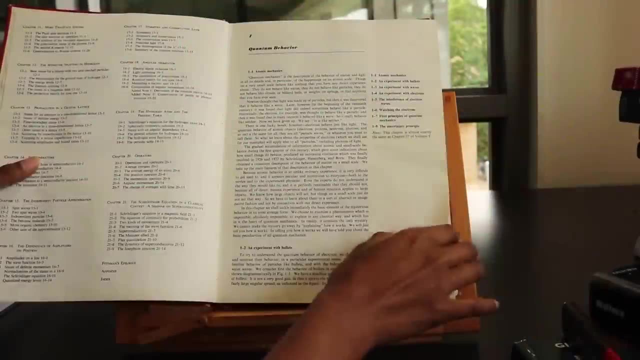 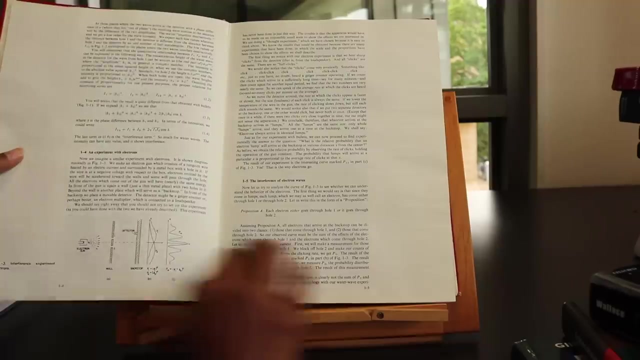 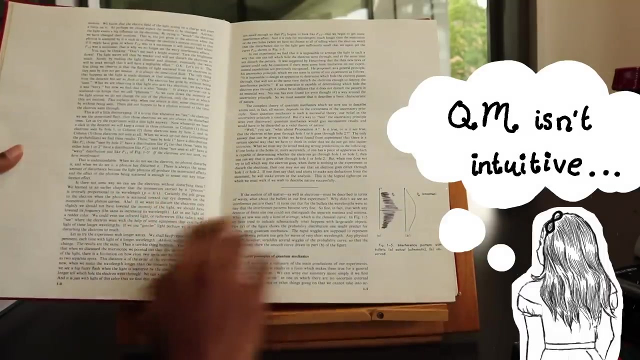 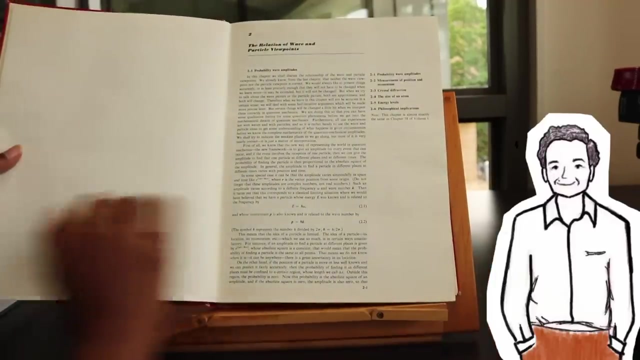 beginners to physics pros. It's volume three of the Feynman Lectures on Physics. You might be thinking: but quantum mechanics isn't intuitive, And that's true. But a good physicist has some intuition for it nevertheless, And Feynman was of course very good. So we're 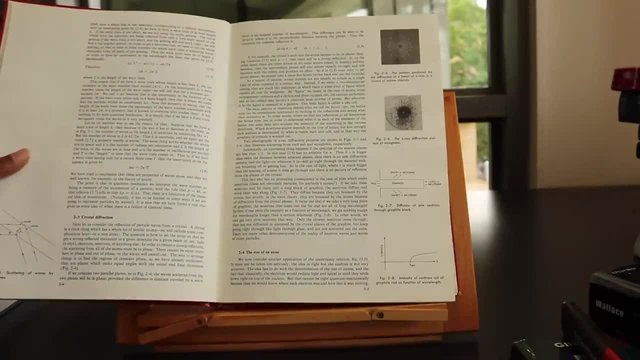 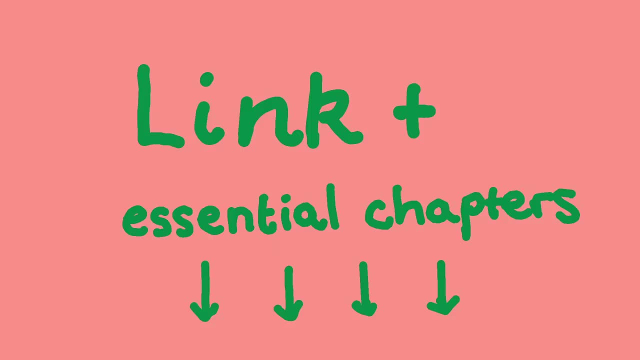 very lucky to have these lectures And, even better, they're free online. So if you're interested in learning more about quantum mechanics, check out the link below. The link, as well as what I think are the essential chapters, are in the blog post linked in the description below. 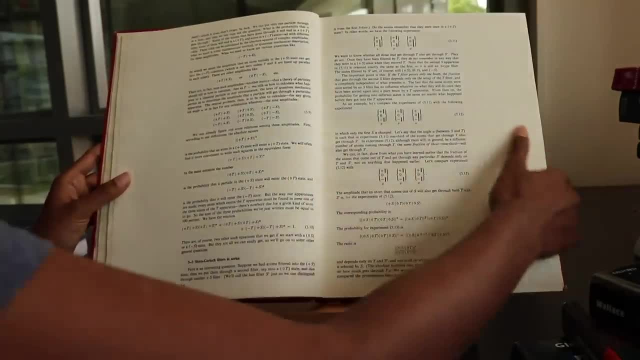 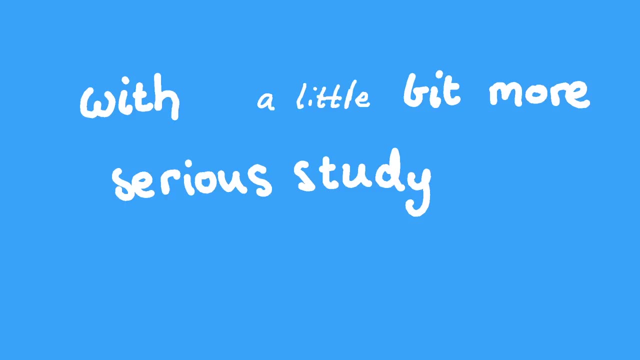 If you don't want to do any more beyond this, then no problem. Reading that alone will give you a very good flavor for quantum mechanics. But if you're willing to do a little bit more serious study, then it really is possible to learn this subject to a very high standard. 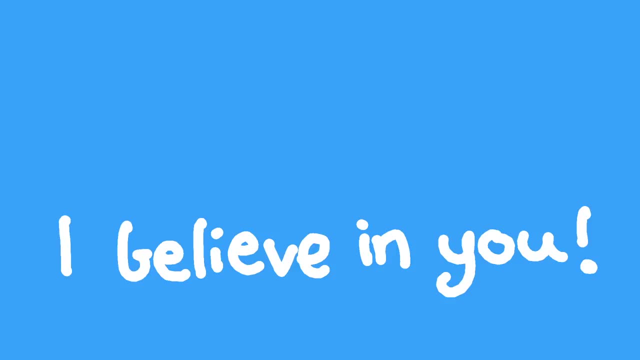 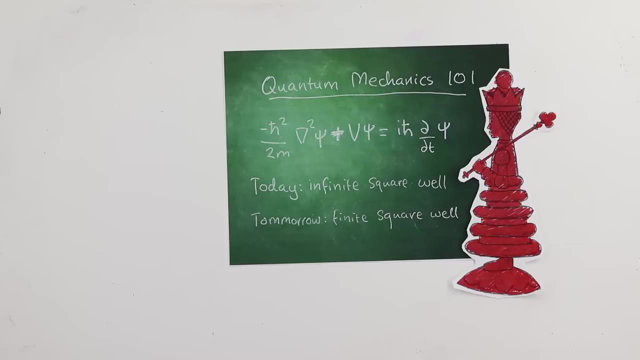 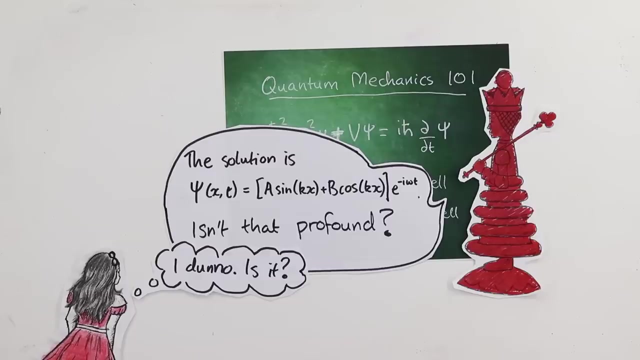 on your own, even without a lot of maths background. See, the usual approach to quantum calculus can be a bit intimidating And even worse, it's really opaque. So it's hard to understand what's quantum because it all just looks like equation manipulation. But the way 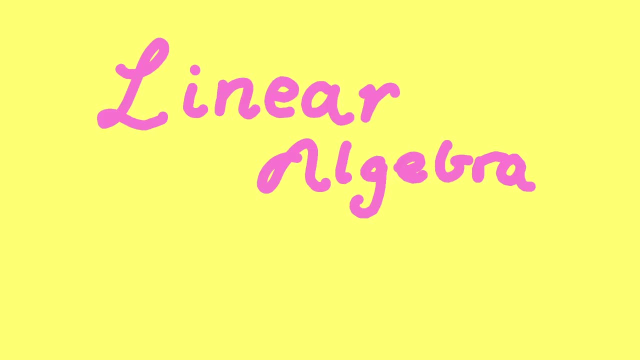 I'm going to suggest, uses something called linear algebra instead, which is, trust me, way easier and generalizes to things like quantum computing much better. anyway, To learn that math background, I recommend a few selected chapters from Gilbert Strang's Introduction to Linear Algebra. 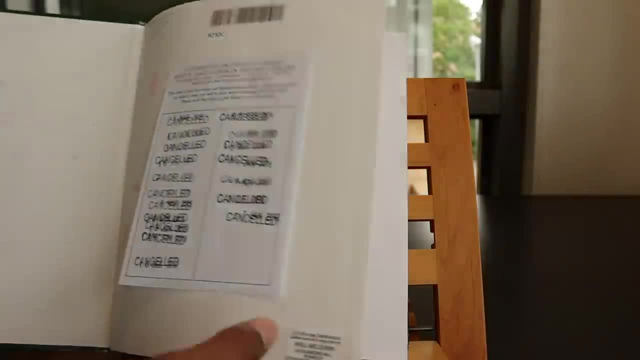 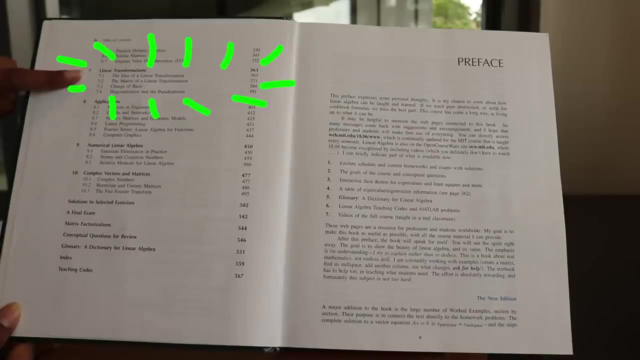 Some of you might already know that topic, but it could be worthwhile to do those chapters anyway, because I find that that material is often not the main emphasis of a standard linear algebra course, And that's why I started making these videos about linear algebra here. I wanted the videos. 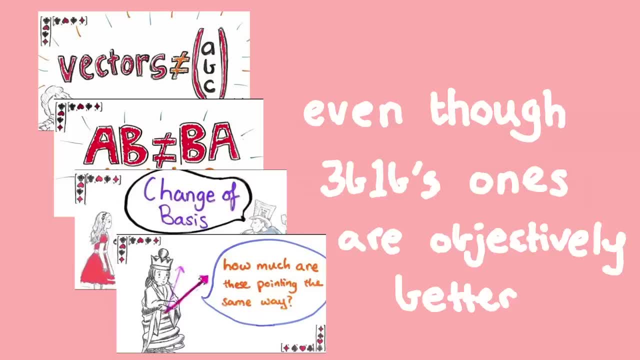 to specifically cover what you need for quantum mechanics. So if you're not sure if you have enough background, watch those videos and see whether you feel super comfortable with those ideas already or not. If you decide to get the book, then try to find the link in the description below. I'll put the link in the description below. 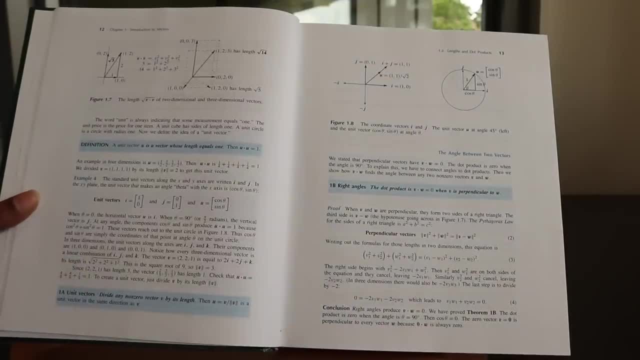 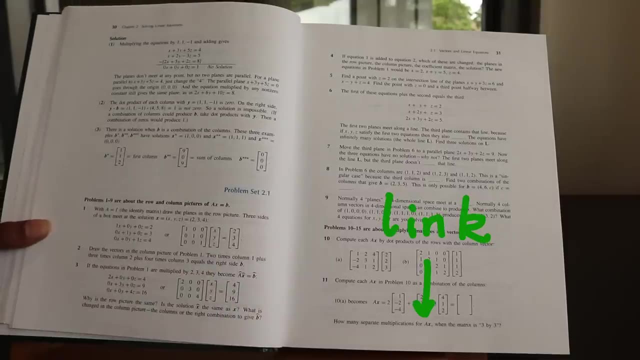 buy a secondhand copy of an old edition. It's a really popular textbook, so there's loads of old ones floating about And there's also free lecture recordings by the author. Anyway, that's the maths out of the way. now for quantum textbooks, I'd recommend two: The 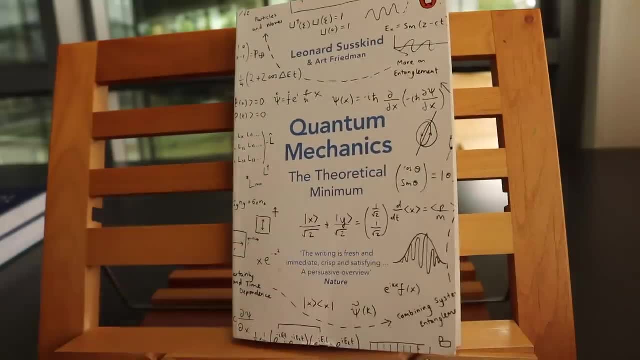 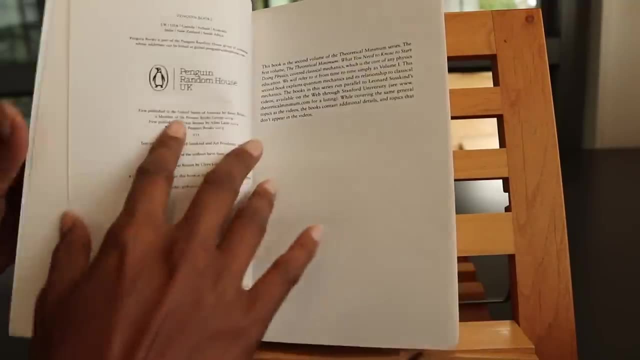 first is The Theoretical Minimum by Landon Susskind and Art Friedman. This book is based on a lecture series that Susskind did for people who wanted to learn quantum mechanics- who didn't necessarily have a physics background. But it's brilliant even if you are a physics major. 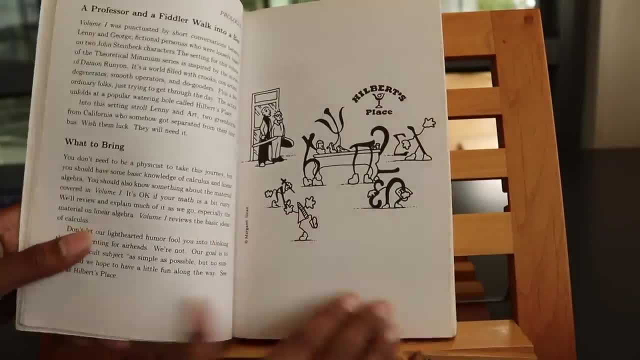 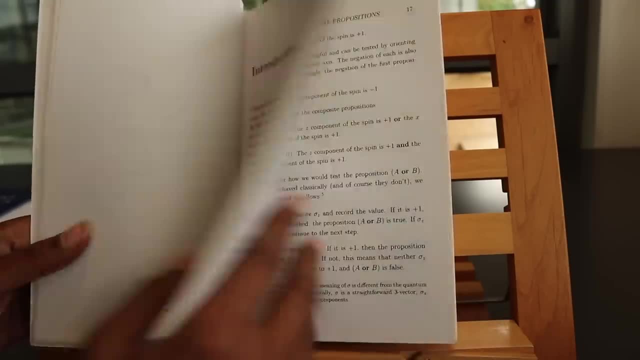 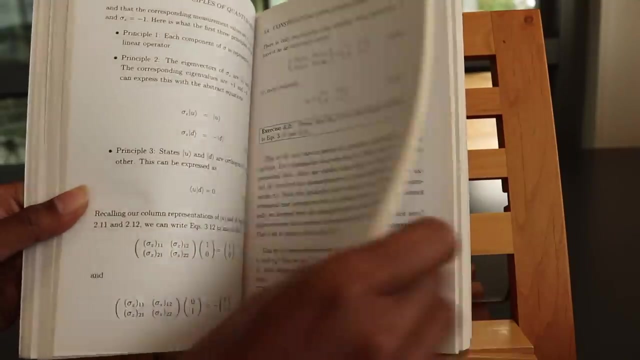 because it includes some helpful discussions before diving into the maths of each topic. Even though it assumes very little knowledge and looks like a novel, don't be fooled: This is a serious textbook that theoretically will teach you as much quantum stuff as a typical undergraduate physics degree. That's why I don't recommend. 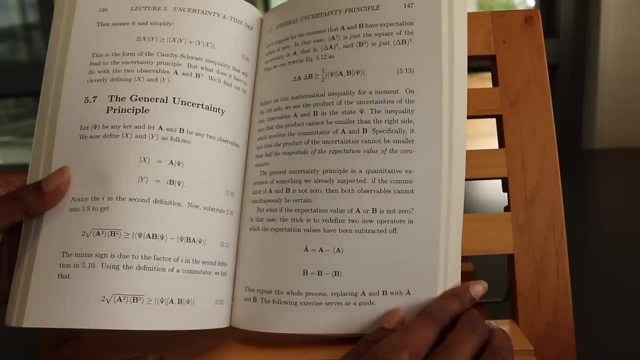 you read it on its own, because it goes from basic to pro very fast. Try reading The Theoretical Minimum by Landon Susskind and Art Friedman. Try reading The Theoretical Minimum by Landon Susskind and Art Friedman. Try reading The Theoretical Minimum by Landon Susskind and Art Friedman. 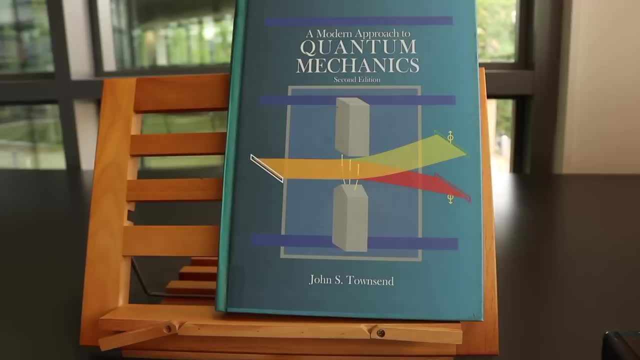 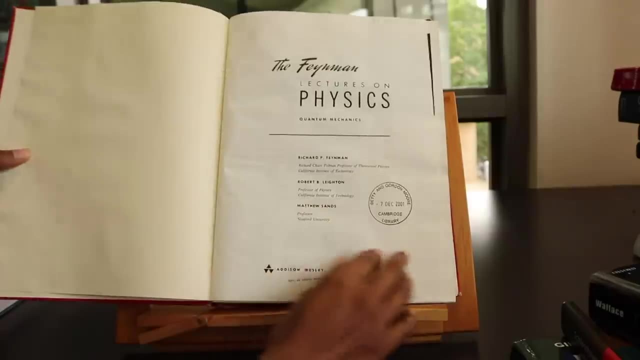 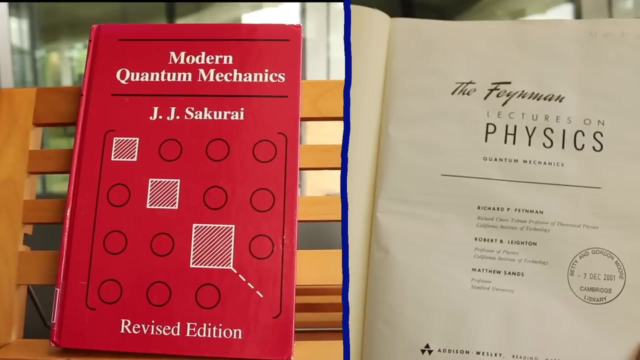 It's one of the few mainstream introductory quantum textbooks that I can really get behind. It's inspired by the Feynman lectures, as well as one of my favourite quantum textbooks, Modern Quantum Mechanics by Sakurai, But Sakurai is basically a graduate textbook. 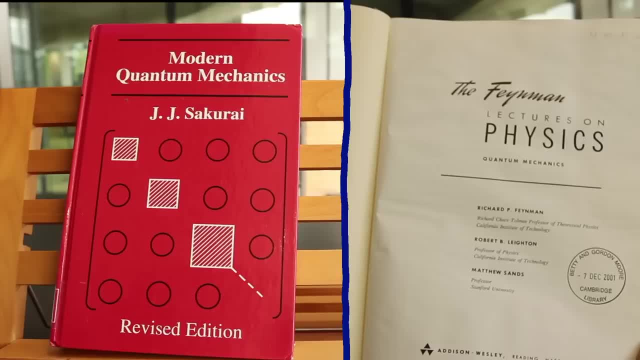 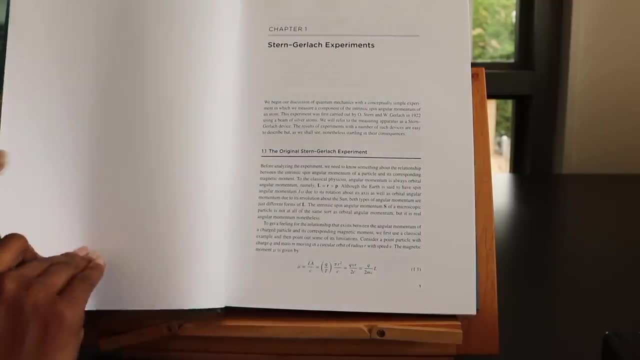 so it's very detailed, and the Feynman lectures are not really detailed enough. so this book captures the core ideas of both at just the right level. It covers a lot of the same ground as The Theoretical Minimum, but in a different way, so I think they complement each. 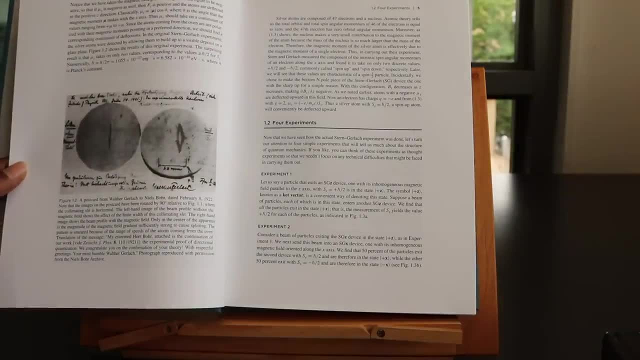 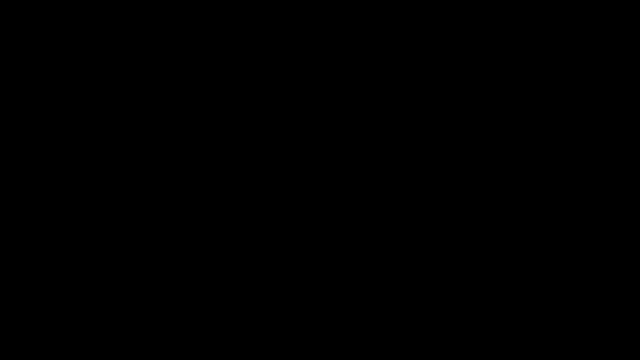 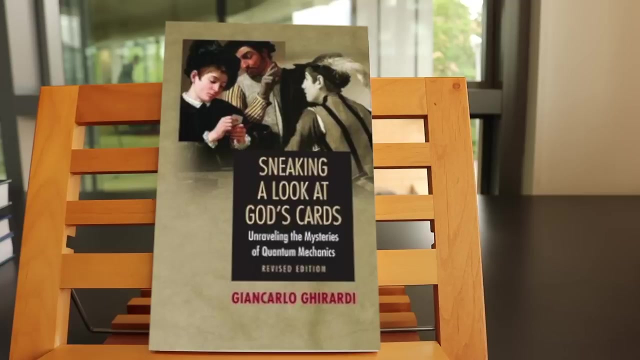 other. What I found was when I was learning quantum mechanics. it's great to see the same thing explained multiple ways. So those are the core textbooks. There's a bunch more I have for advanced topics that you might be interested in reading after these three or if you've done quantum mechanics before, but I'm going to talk about. 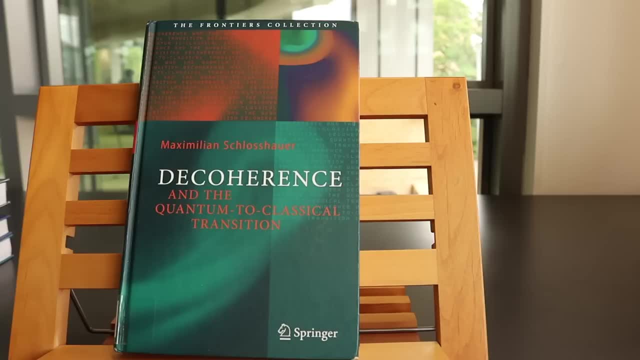 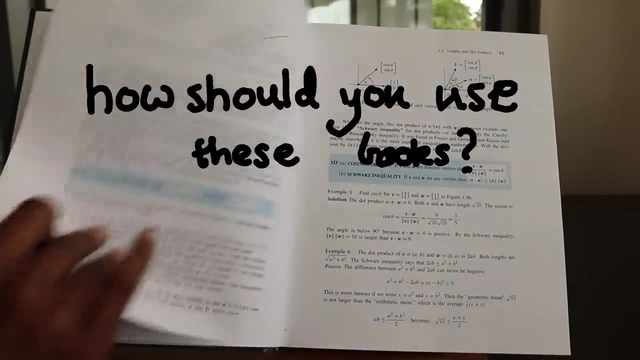 them in the blog post instead of here. How should you use these books, though? It's really easy to trick yourself into thinking that you understand maths or physics when you just read and re-read a textbook and look at worked out solutions. But, as Scott Young explains in his new book, 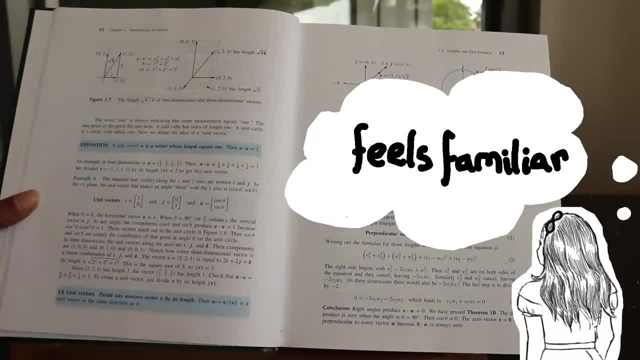 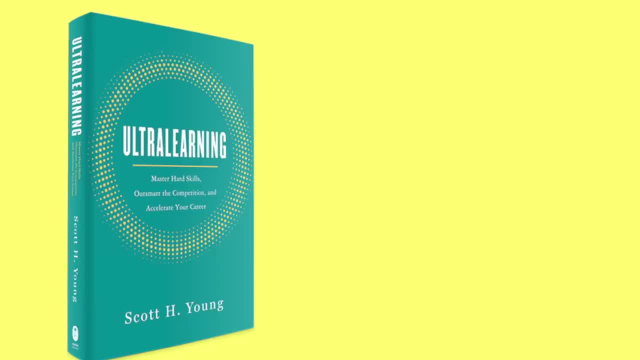 about learning. what's really happening is you start to feel familiar with the text, but that's very different from understanding it. In his book, he gives a whole bunch of different methods to get around this and other issues you might get stuck on when you're learning. 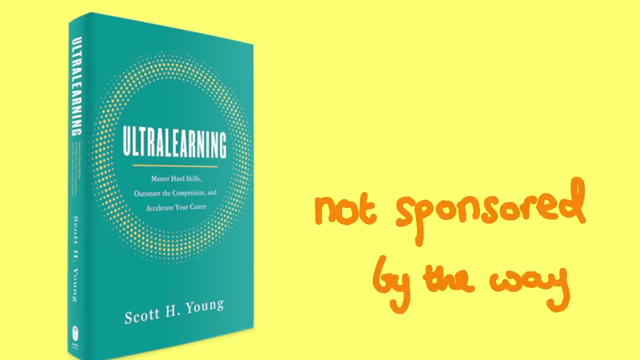 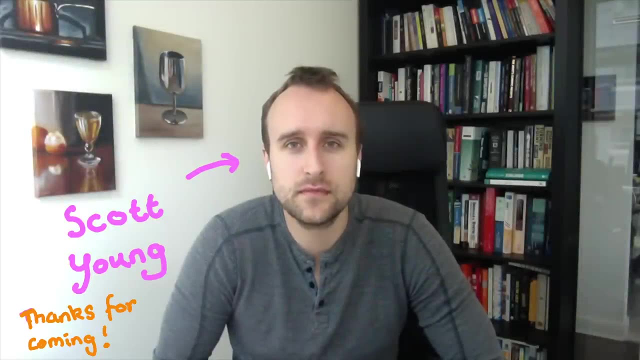 something on your own. I seriously enjoyed the book, so I decided to ask Scott what tips he'd most recommend for you guys for this specific project. Here's what he said. Well, the most important thing is to just do a lot of practice. I think that a lot of people 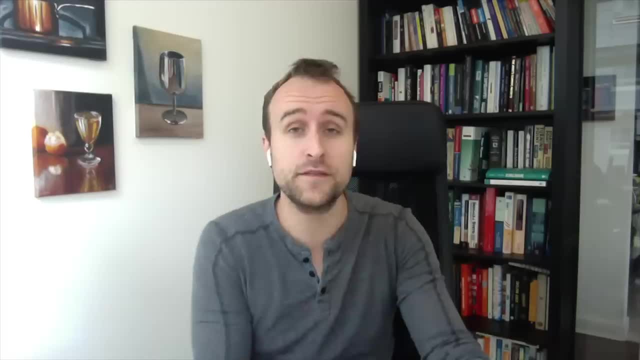 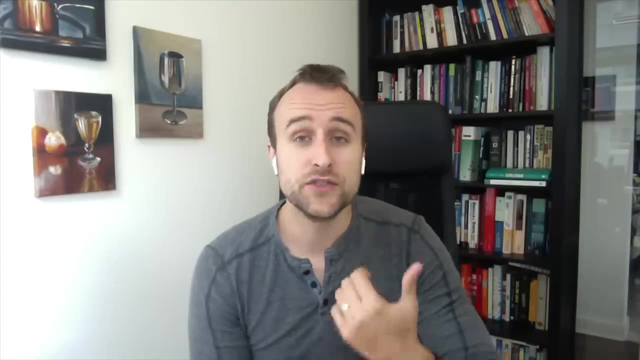 get the idea that the main way that you learn something like physics is by attending the lectures and reading the textbook, But I think that the main way you learn it is actually doing the practice problems. The first reason this is more effective is something known as retrieval. 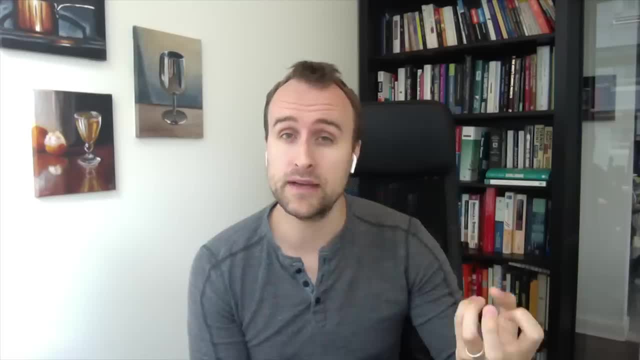 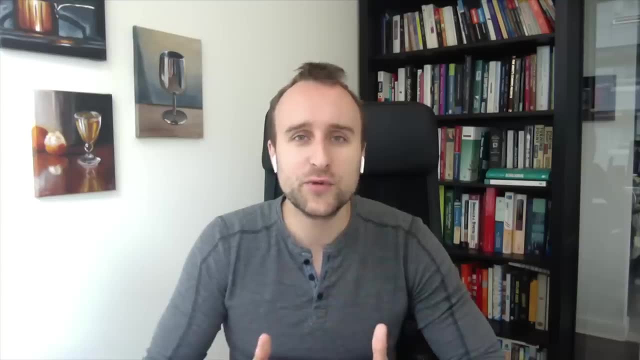 So retrieval is the idea that if you actually have to practice remembering something from your head, you'll be much more likely to retain it than if you don't, if you just passively review it looking over your notes. The second reason is that physics is a skill, Just as you wouldn't learn to ride a bicycle by. 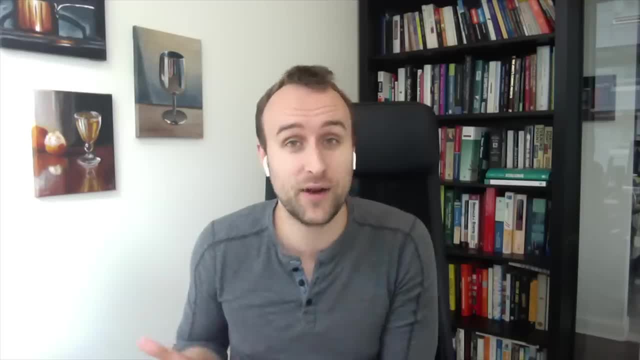 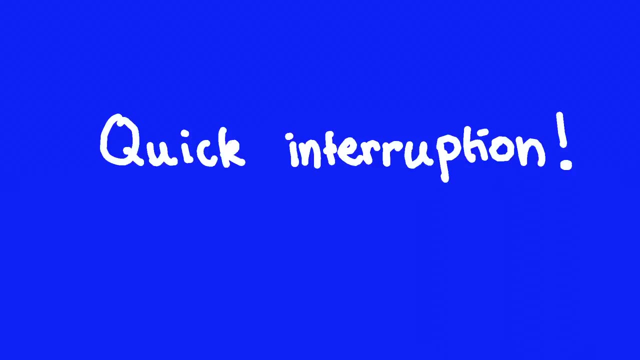 reading a book on learning to ride a bicycle, but by actually riding a bicycle. similarly, if you want to be able to do physics problems, you actually have to do physics problems. Quick interruption here. I couldn't agree more with this point, and so in the blog post I've marked what problems you should be. 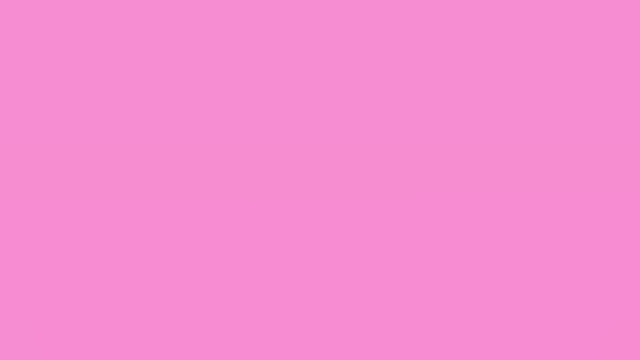 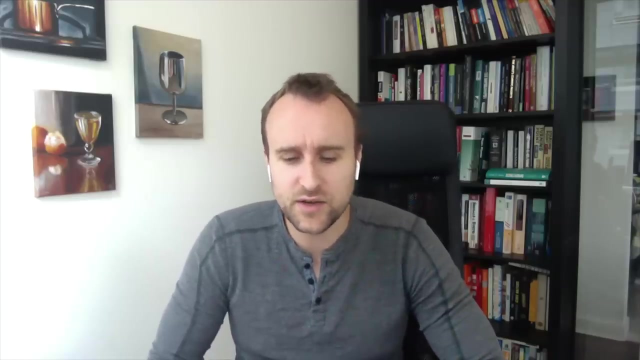 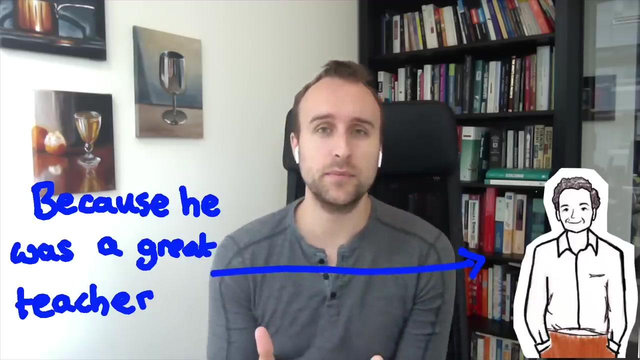 doing with the texts I recommended, including for the Feynman lectures. So the Feynman technique is a method that I developed about ten years ago and it was named after my real inspiration in learning hard things, Richard Feynman. So the method is really simple. Basically, you just take a sheet of paper. 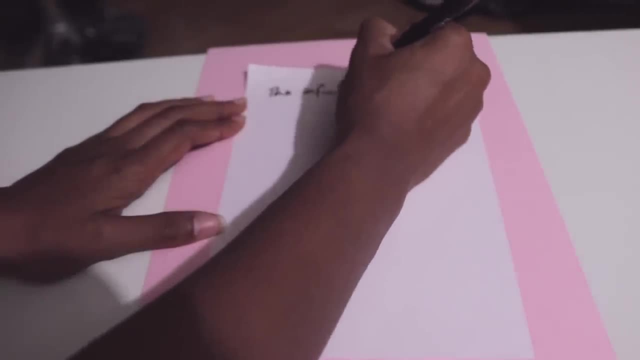 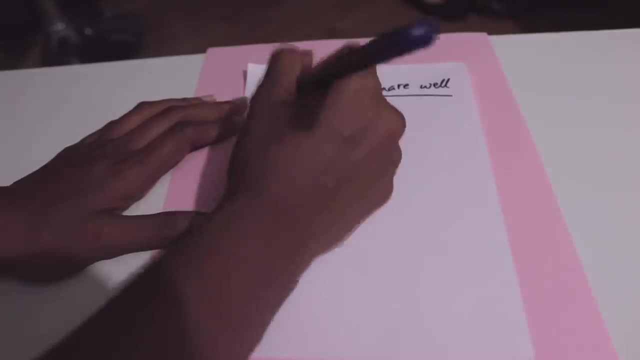 and you write down the thing that you don't understand at the top. So it could be understanding torque or understanding the infinite well problem in quantum mechanics, And then you go through there and try to explain the problem to someone else as if you're teaching it. 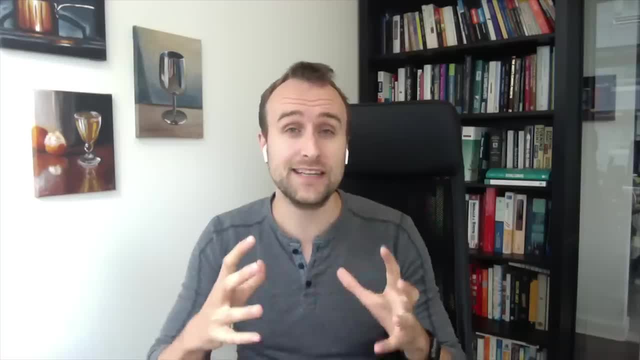 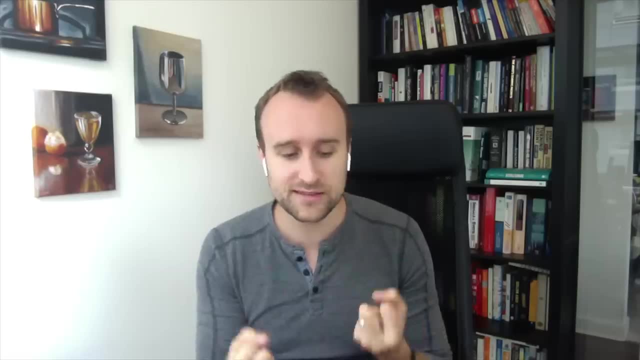 So the The thing that this is really helpful for is that, first of all, it takes all of your thoughts, all of your confusions, and puts them on the paper. So suddenly, when you have things on the paper, you can sometimes figure out the answer that 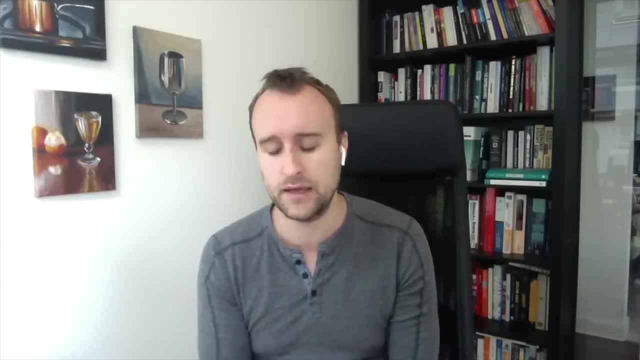 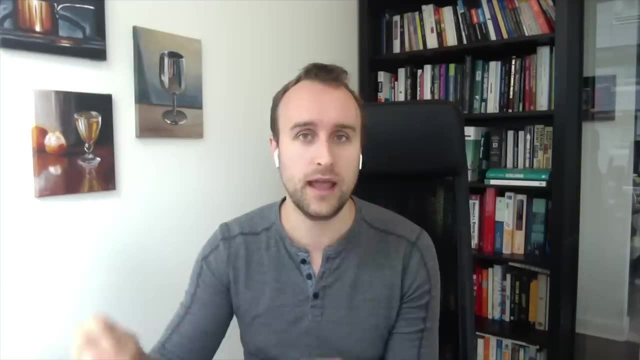 you were missing. Oh, this is what I didn't understand, just by putting it on the page. The second reason that this is valuable is that it allows you to slow down your process through a particularly difficult point. So a lot of physics is really confusing, and it can just be a situation where you're like 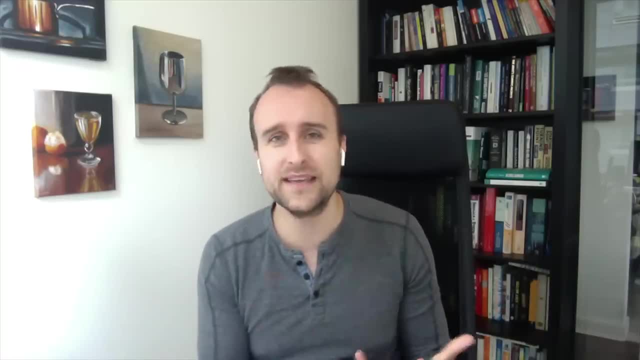 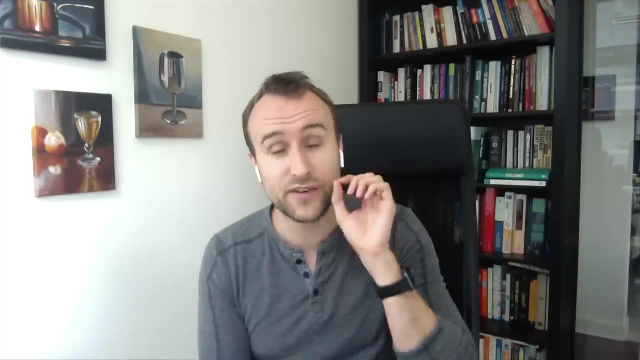 I don't get it and you throw your hands up And that's not very helpful, because just I don't get it doesn't really give you any obvious road forward, Whereas if you slow it down, you can start by asking yourself very specific questions. 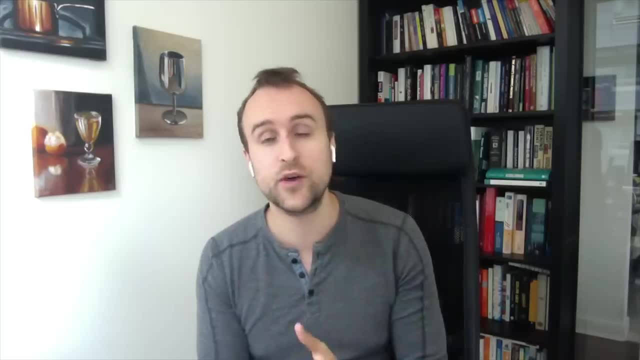 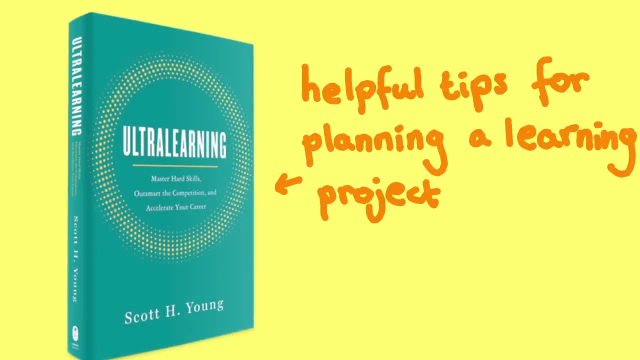 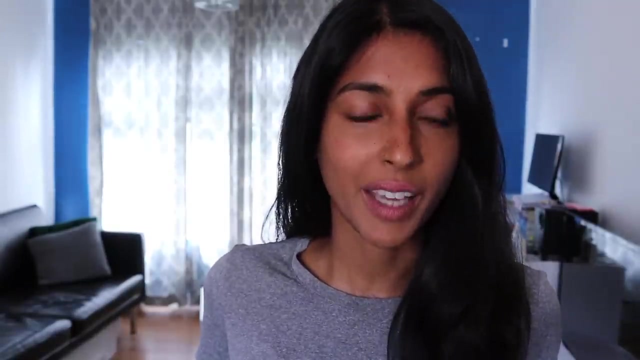 What exactly don't you understand about it? And when you have very specific questions, it's much easier to look for very specific answers. If you want more helpful tips about learning from Scott, I highly recommend his book Ultra Learning. The Feynman technique especially resonated with me because that's how I learned quantum. 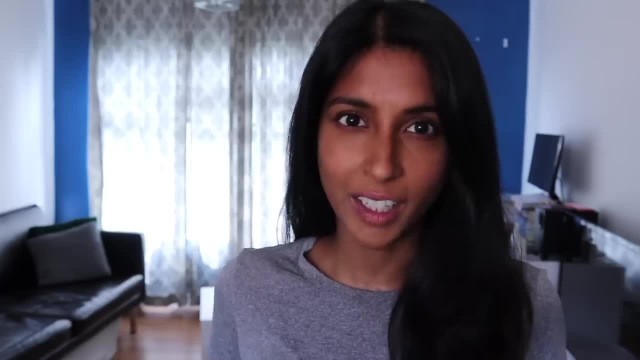 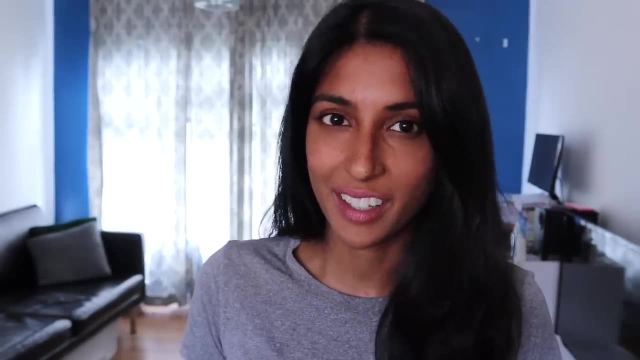 mechanics. I would read textbooks and then, when I felt like I'd got it, I would try and explain them in YouTube videos. these YouTube videos, and that's how my channel started. The thing is, when you're trying to explain something to someone, there is no hiding what. 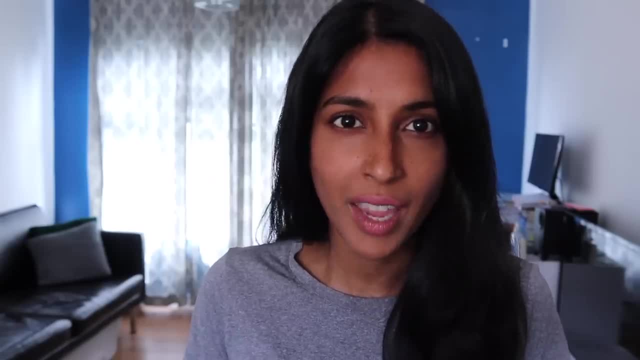 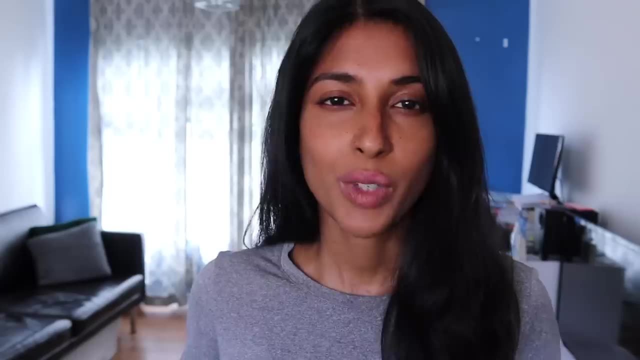 you don't understand. And also, when you want to convey an idea to someone, you want to give them the core intuition, and so it forces you to come up with that core intuition. Once you feel like you understand something, try and explain it, but try and explain it. 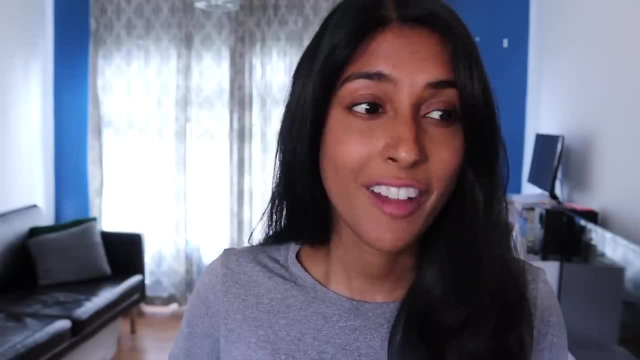 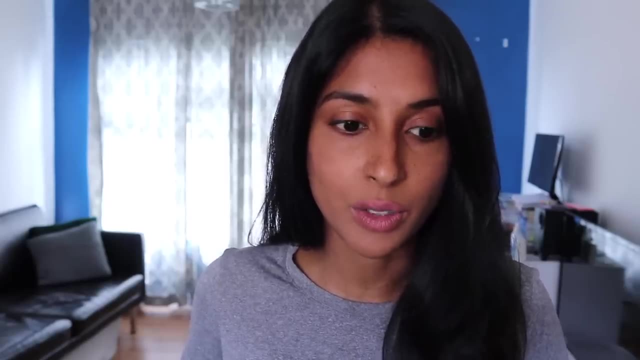 without any jargon or difficult equations. What I found doing this is that it's a lot harder than it seems Like. when I would be going through a textbook, I would feel like I understood everything and I could follow all the arguments. but as soon as I had to explain it without the mathematics, 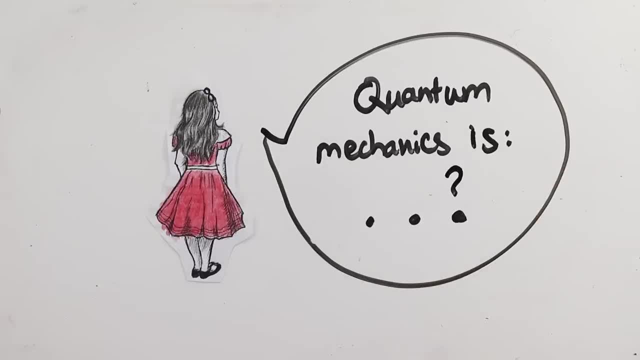 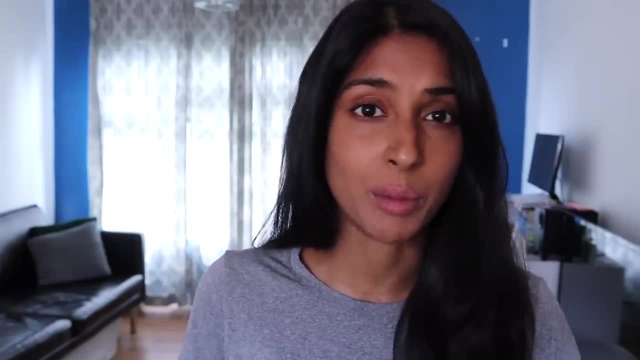 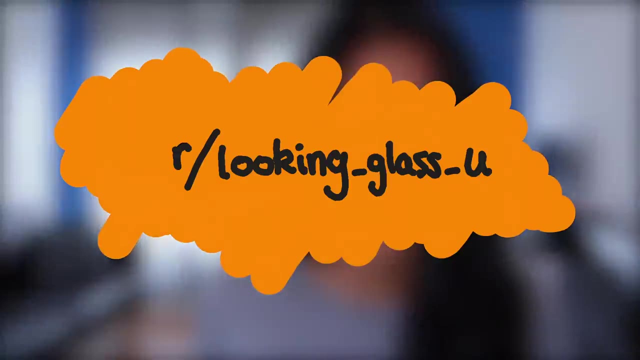 I realized that I didn't actually know what was going on underneath the equations. Now, if any of you do end up making videos or writing articles or, in general, if you just end up doing this project, I would love to hear about it, And so I've finally made a subreddit for this channel where you can keep me up to date.